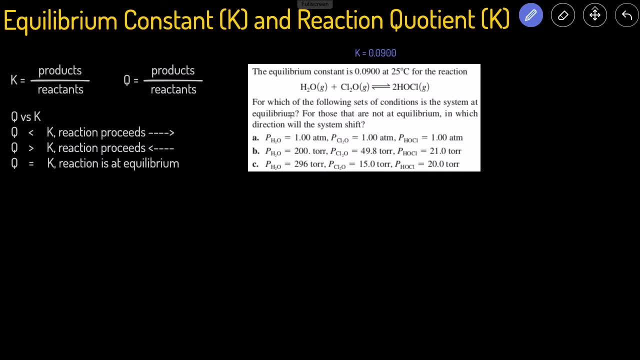 balanced. And then it's asking us for each of these conditions: is the reaction at equilibrium? And if it's not at equilibrium, in which way will the reaction proceed, to the right or to the left, to reach equilibrium? So, whenever you're asked about what are reactions at equilibrium and which 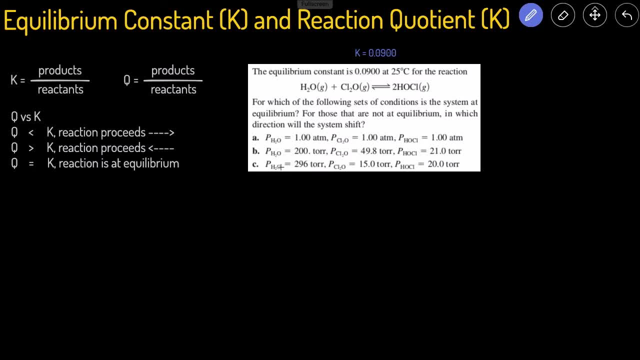 way the reaction will proceed. that's a class indicator that you're going to be comparing Q versus K. So we have the K value. Let's start by writing the Q expression so we can start to calculate the Q value. So we know that Q is equal to products over reactants, But this time they 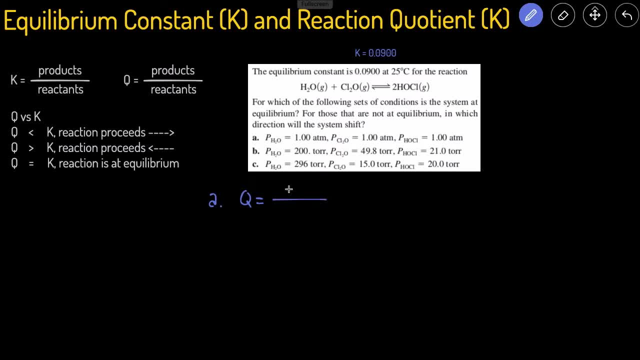 give us the pressure. So we'll be using pressure products over pressure reactants, So we'll have pressure of the HOCl And there's a coefficient of 2.. So that means we got to square this, because the coefficient become the powers divided by the pressure of the reactants And they're both gases. 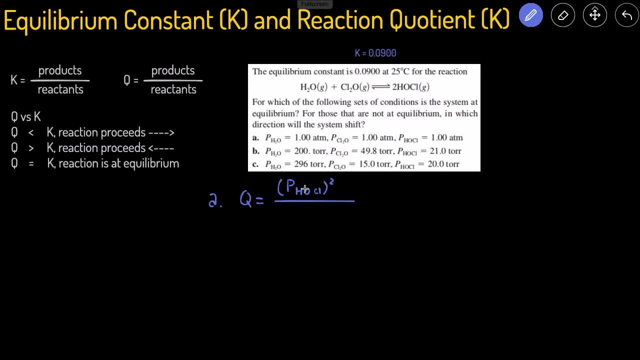 We want to check the states, because we never include solids or liquids in the Q or the K expression. All of these are gases, so they're all fair game. Then we have pressure of H2O on the bottom, raised to the coefficient- There's a coefficient of 1, so raised to the first power times the pressure. 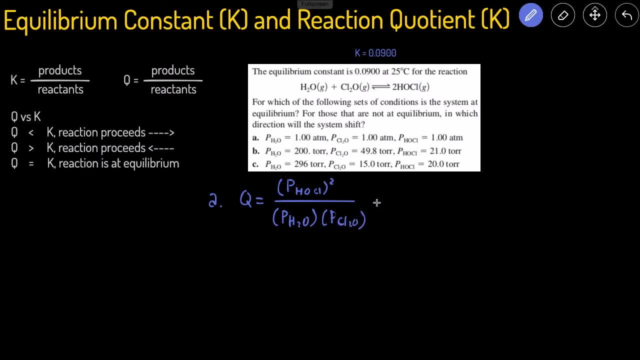 of the CO2O also raised to the first power. So now that we have the Q expression, let's plug in the values. So the pressure of the HOCl is 1.00.. And we're going to square that. divide it by the Q expression and we're going to square that. 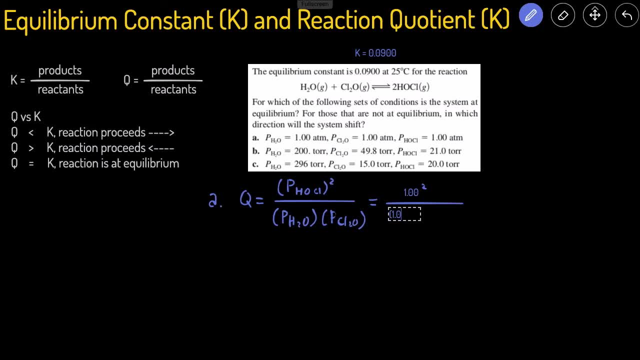 We're going to square that by the pressure of the H2O, which is also 1.00,, times the pressure of the CL2O, which is also 1.00, as you can see right here. So this is going to be 1 divided by 1.. So that means 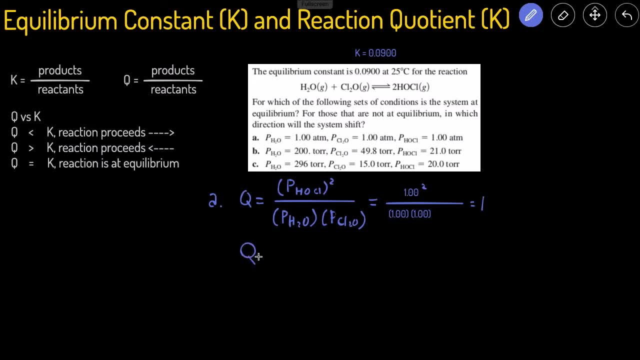 that our Q value is 1.. So our Q is equal to 1.. The K was equal to 0.0900.. And then you can see that the Q is greater than K, which means the Pac-Man is eating to the left. So that means this reaction. 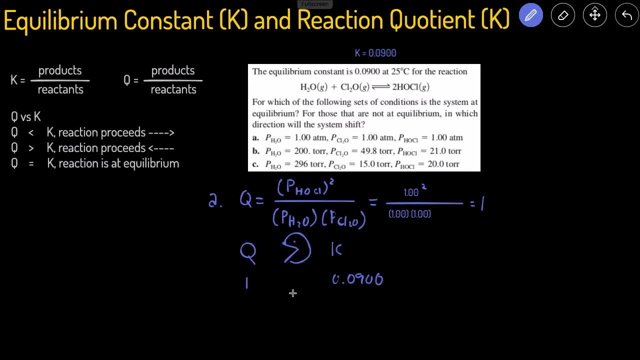 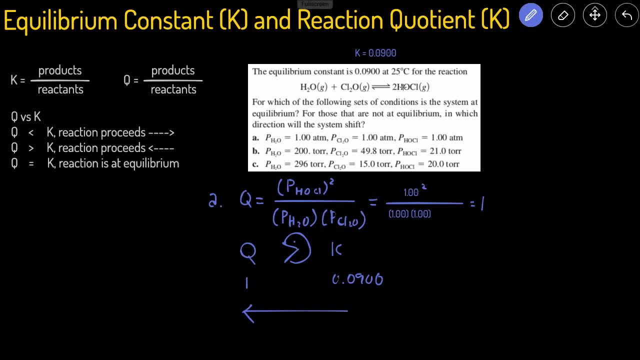 going to be producing more reactants and then we're going to be consuming the amount of products. So that's how we do A. So for B, it's the same approach, but we're just going to switch some of the numbers out. So let's recalculate the Q for B: The pressure of the HOCl, the product is 21.. 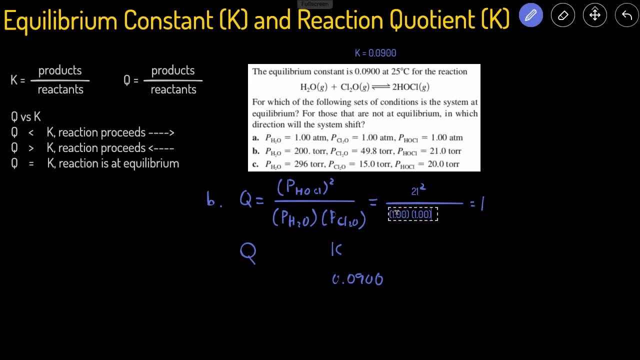 and then we have to square that. the pressure of the h2o- it's 200 times the pressure of the other reactant, cl20, is 49.8. let's plug that into the calculator and see what we get for the q value, and then that gives us 0.044. so now plug that back over here: 0.044. you can see that. 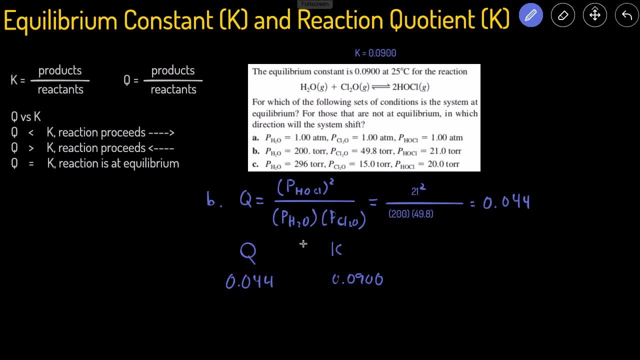 the q value is less than the k value this time. so that means that the pac-man is going to be eating to the right, which means that this reaction is not at equilibrium and that the reaction will be shifting to the right to reach equilibrium. so we'll be producing more products and consuming. 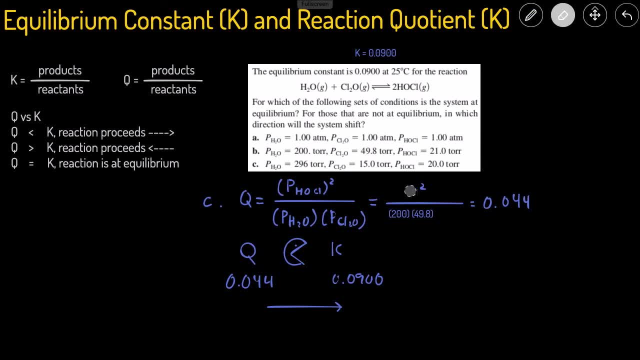 the reactants. all right, now let's take a look at c. so for c, the cons, the pressure of the product was 20 and we got to raise it to the second power. we got to carry this two over, divided by the pressure of the reactants. 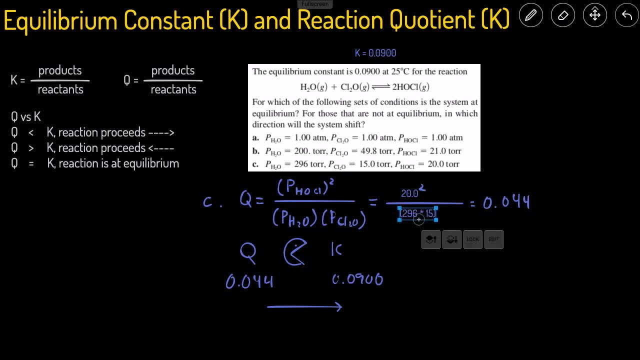 296 times 15.. and then that gives us 0.00900. and so now we have a situation where the q is exactly equal to the k. that means that this reaction is already at equilibrium, and that's the main purpose of using the q versus the k. again, q and k, they have the exact same. 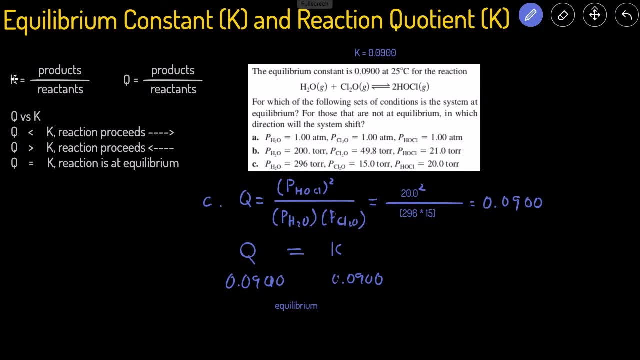 expression, but k refers to the equilibrium constant, which is not changing if the temperature is constant, whereas q is going to change as the reaction progresses. you can use q versus the k to determine if a reaction is at equilibrium and if it's not, it'll tell you which way the reaction will shift to reach equilibrium. if you want to learn.